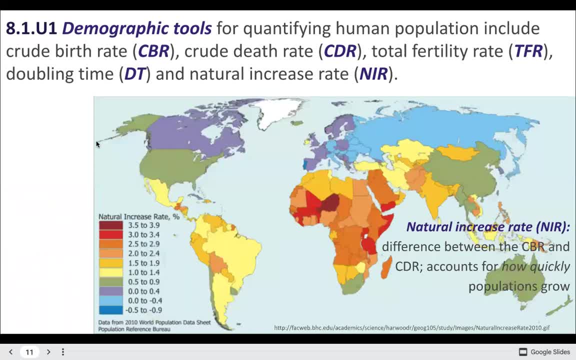 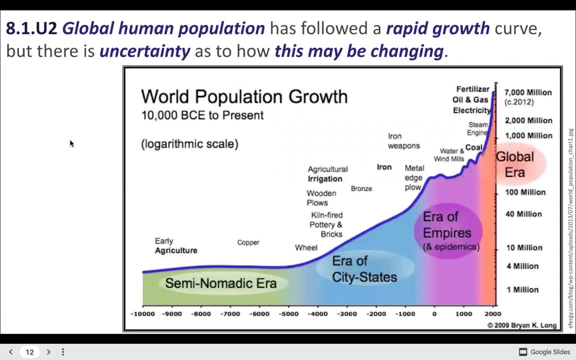 these again, But I've usually seen like maybe one or two questions about this on exams. Like you know, calculate the doubling time for such and such Global human population has followed a rapid growth curve, but there's uncertainty as to how this is changing. So back in the 1970s, 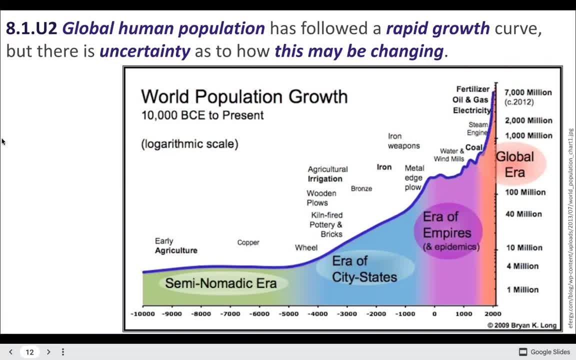 they're like talking about the population bomb and like, oh my God, we're totally screwed, We're gonna have way too many people. And then they're like: oh my God, we're totally screwed, We're gonna have way too many people. This is a really funny scale, because we're going like 1 million. 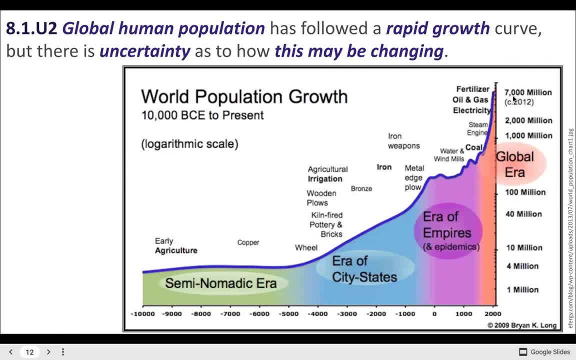 4 million, 10 million, 100 million, 7,000 million. I don't know about this scale. It's logarithmic. I'm gonna argue about whether or not you think this is a useful scale to use, But I guess it. 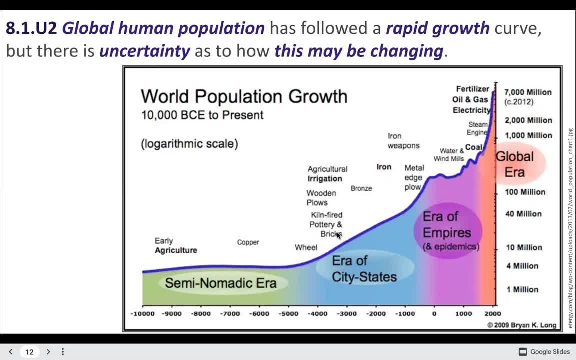 kind of shows like when you have a larger population it's easier to grow faster. So this sort of shows that maybe our population growth has been relatively consistent until maybe very recently. So that's a lot of people talking about. oh my God, the population bomb like there's too many. 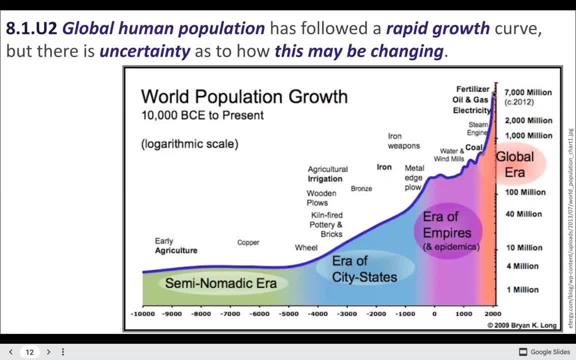 people. That's sort of based on old information about reproduction rates, And most countries in the world have a reproduction rate of just around two- a little bit over two people per couple. So that's basically replacement rate right. So we're probably fine As human population grows. 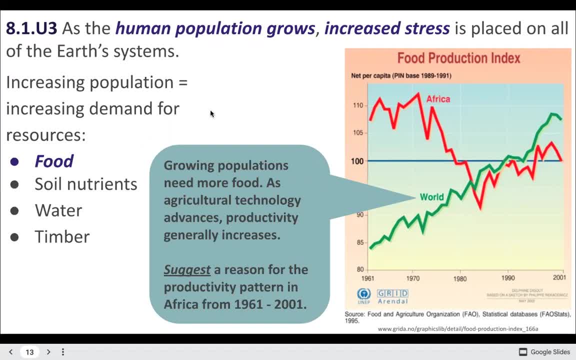 increased stress is placed on all the earth, So we're probably fine. As human population grows, increased stress is placed on all the earth, So we're probably fine. As human population grows, increased stress is placed on all the earth, So we're probably. 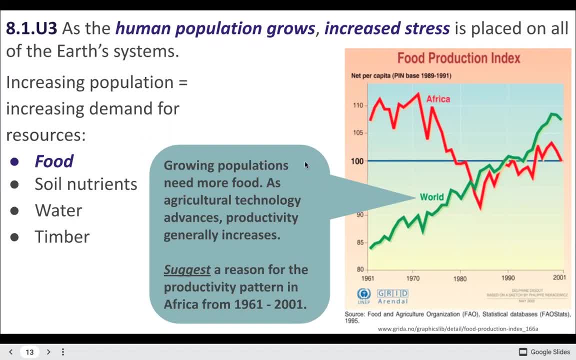 fine. As human population grows, increased stress is placed on all the earth, So we're probably fine: Food, soil, nutrients, water, timber. It's really worth pointing out that, like different populations use different amounts of resources, And sometimes I feel like it's unfair just to say increasing. 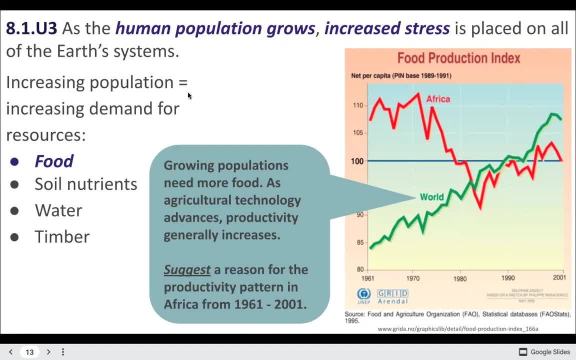 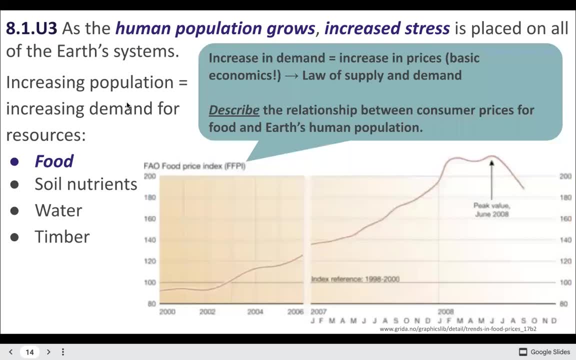 population equals increasing demand, Because you can have an increasing population that has a much smaller ecological footprint and that could make a lot less of an impact. you know, It's really all about how you're living, not just how many people are living. It's pretty important. 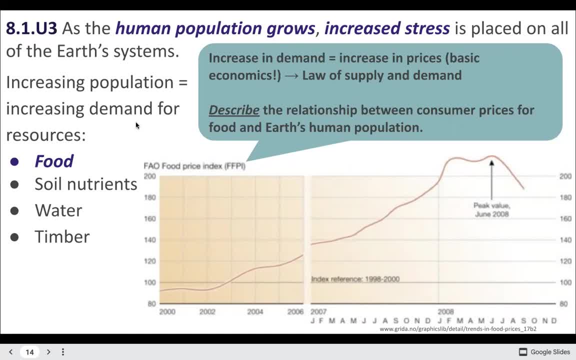 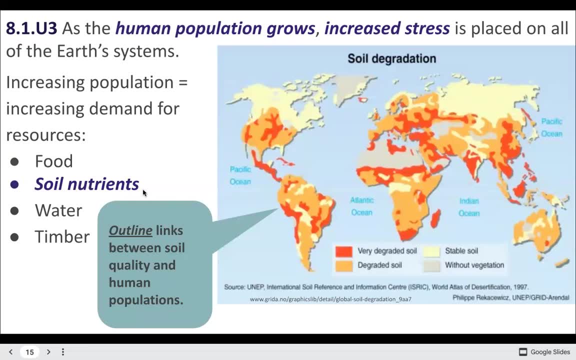 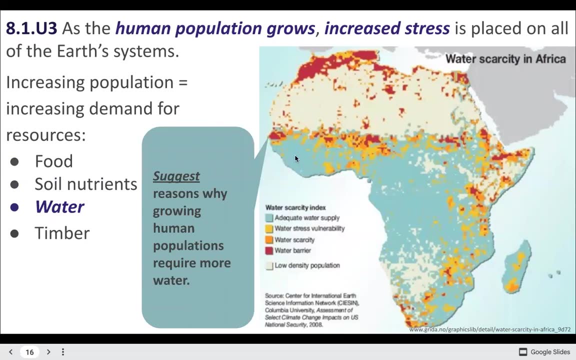 It's pretty unfair to just say it's because of the number of people, when some of them use way more resources than others. Okay, So increased stress on things like soil nutrients: right. So increased stress on water. We have lots of water conflicts around the world. Increased stress on other natural resources. fossil fuels, etc. And as we have more urban populations, we have to, you know, support them by building all the cities and then getting all of the resources to those cities and providing them with clean water and shelter and everything else. But yeah, cities are pretty good for concentrating populations and for lessening. 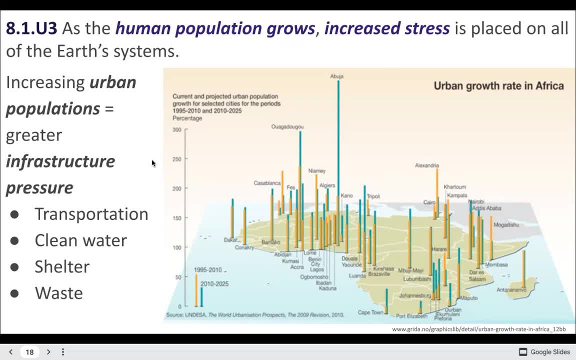 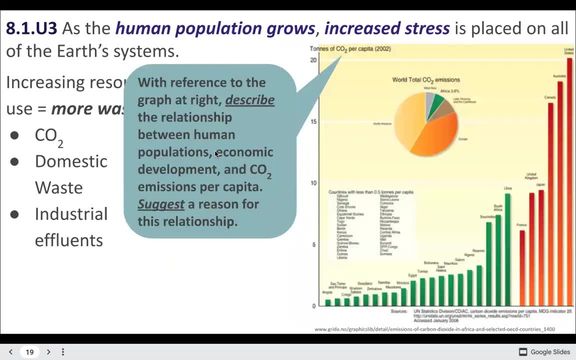 impact elsewhere. You can make really sustainable cities that are really population dense and then conserve a lot of wild spaces. There's this like super interesting concept by David Brower, who was the president of the Sierra Club And he's actually the one that gave up Glen Canyon and felt really bad about it after he gave it up. 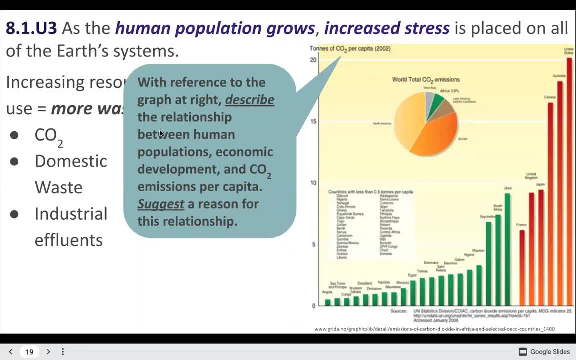 But he wrote a book and one of his proposals. he's like, basically like right now we have national parks and we have wilderness areas and we like build walls and fences around these wilderness areas, And so his argument is that we should switch that and we should start. 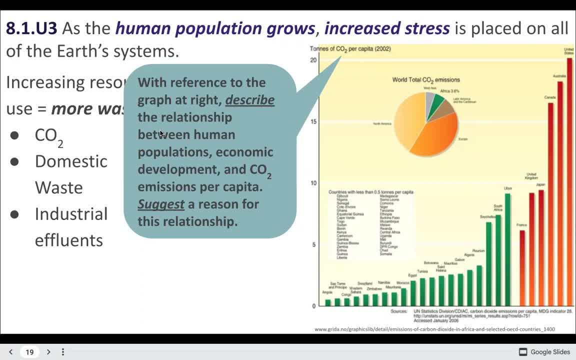 building walls around our cities and concentrate people in cities And then sort of let the rest of nature be wild and free And then we're sort of containing people in areas where they are not making an impact. Be pretty wild if that ever happened. 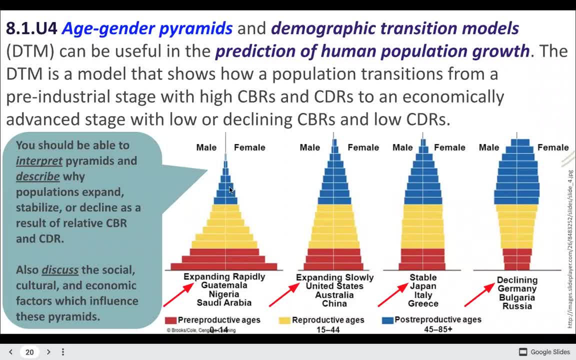 I'd be surprised. So we can look at age, gender pyramids and demographic transition models to see how countries are changing. So, as we mentioned before, Japan is actually over here, where they have a really, really small young population and a lot of folks who are in the middle of the country. 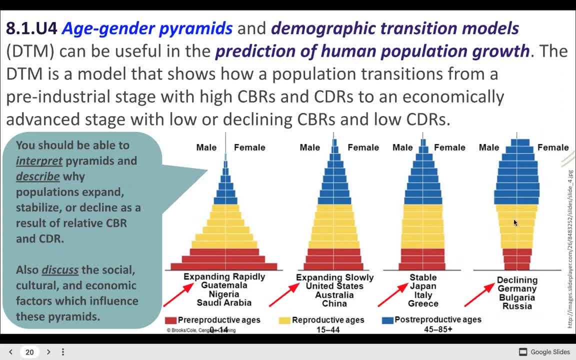 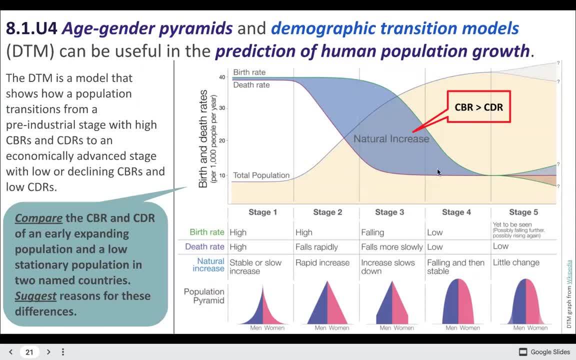 Folks that are entering retirement, And so the big issue here is that how are they going to support all the young people? I have another full video where I go through all of these stages, so I'm not going to go into too much detail here. 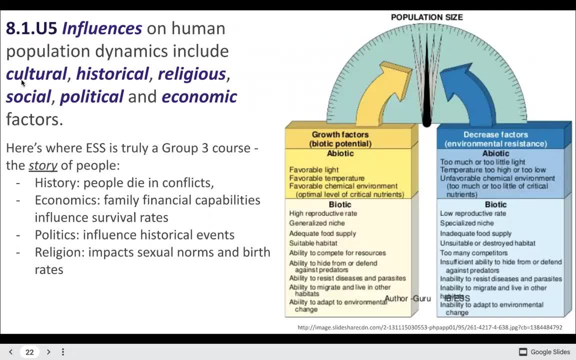 But influences on human population dynamics like pretty much everything, could be cultural, historical, religious, social, political, economic, etc. You might hope that we're just making population decisions based on logic and reason and trying to be environmentally sound, But it's hard to argue that religious aspects don't come into play. 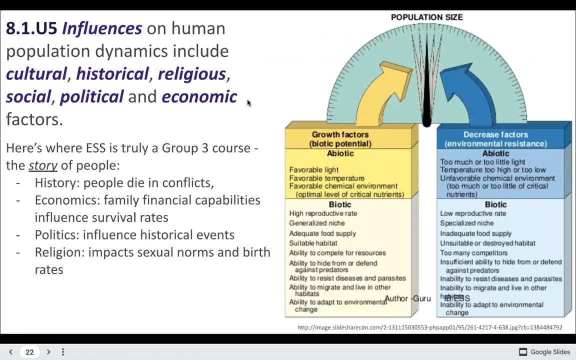 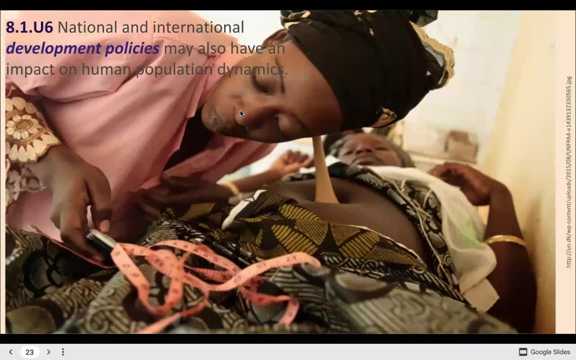 that economic aspects don't come into play. A lot of different reasons that people might have more or fewer children, So national and international development policies may also have an impact on human population dynamics. Really cool in Malawi to see all the efforts done at like getting sort of like midwives and having people provide child care for childbirth and kind. 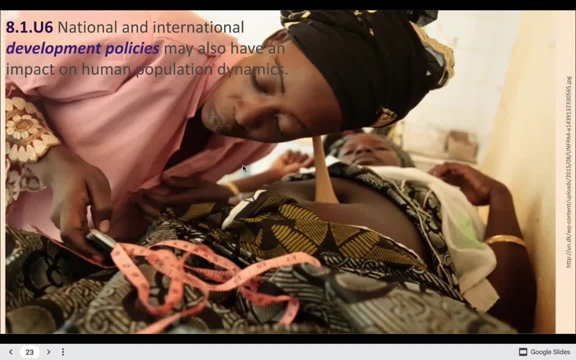 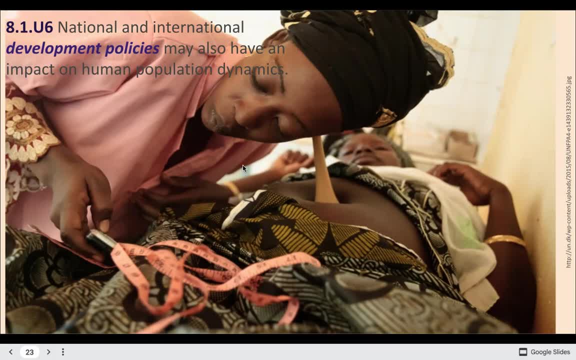 to get to a hospital. When we were in Malawi, a woman walked three miles to give birth at our birthing center, which was not a hospital and which would have technically been illegal, But that was already three miles right. The hospital itself was probably 20,. 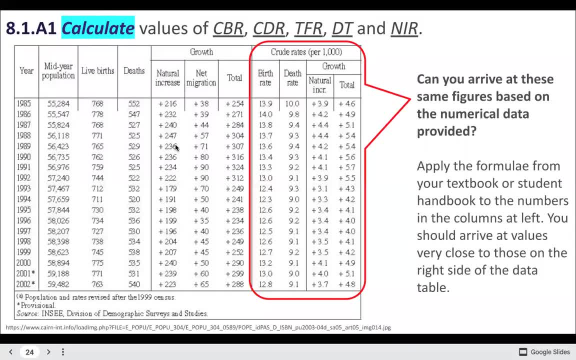 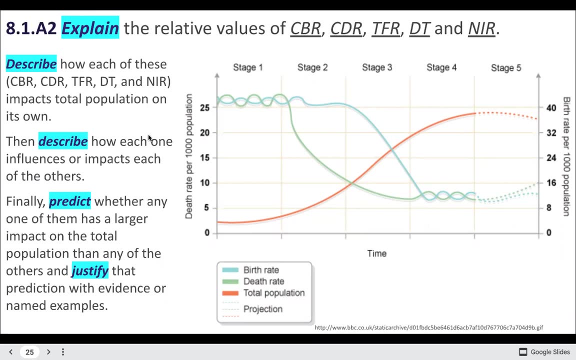 30 miles away. It's like just totally unfeasible. So if you want some practice, you could try calculating some CBR and CDR and TFR and DT and NIR. if you really want to. You should be able to explain the relative values, what they mean, how they can affect. 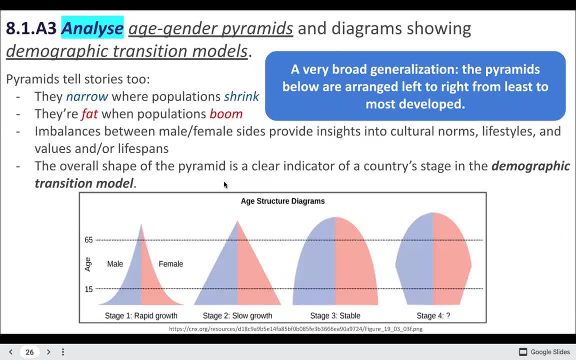 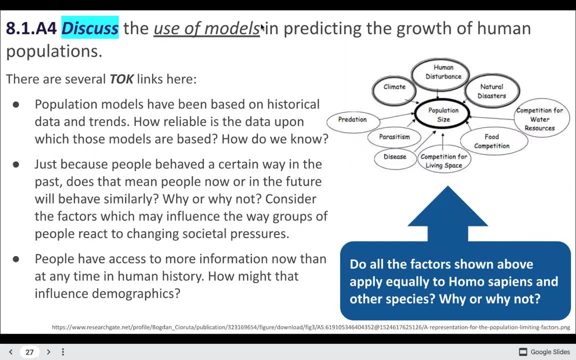 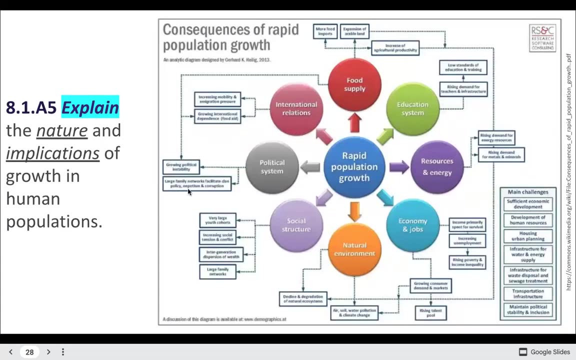 the total population. You should be able to explain, like, how those trends are changing over time, right? The demographic transition model overall, right? That's an example of models which predict how our population is going to change. Cool, cool. You should be able to explain. 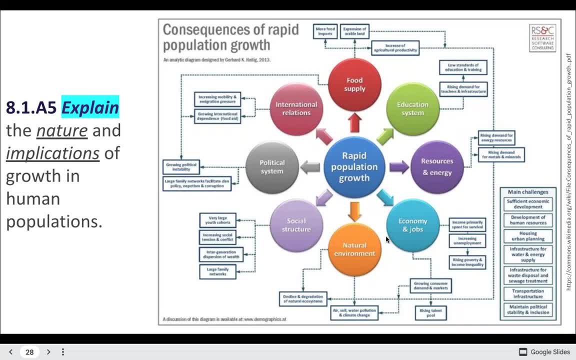 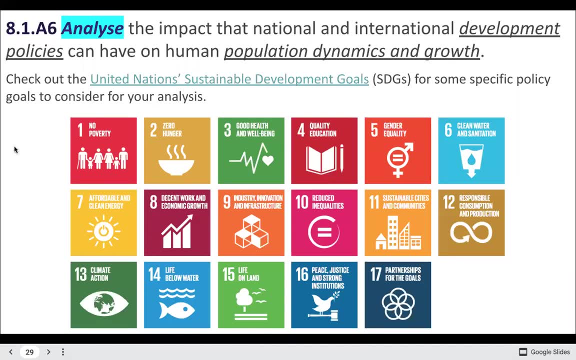 the nature and implications of growth in human populations. More people, more resources. We need to give them food. We need to have a political system. You should analyze the impact that national and international development policies can have on human population dynamics and growth. 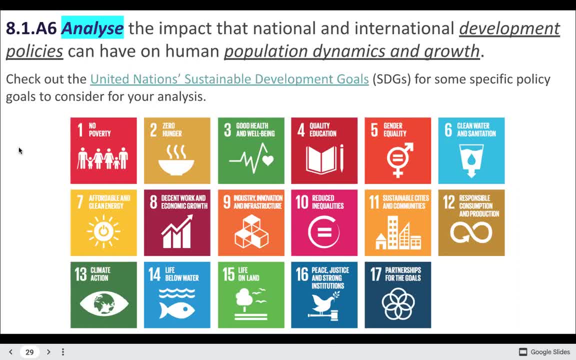 Hey look, it's the sustainable development goals that Caroline is always talking about, that we really try to focus on at our school, And you'll probably notice a lot of connections to ESS in here. right, I got some topic five stuff. We got some topic four stuff. We got some topic two and three.